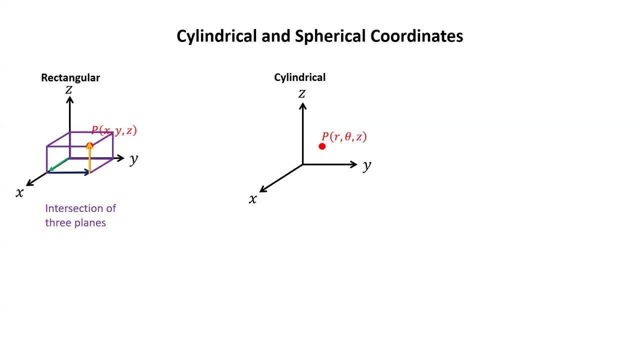 And the z-coordinate z is the same as the z in rectangular. We're moving perpendicular to the x-y plane to get to z. We could think of that point as lying on a cylinder, where from the origin we come straight out r units in the x-y plane, making an angle of theta with the positive. 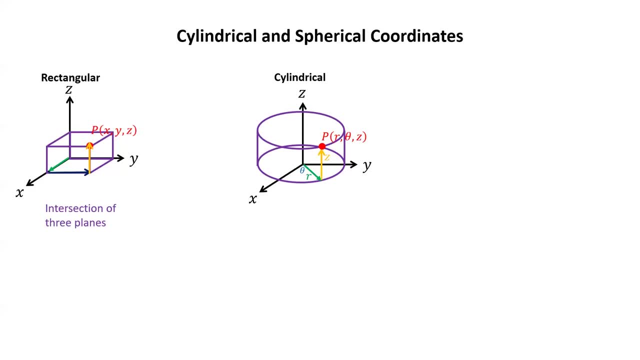 x-axis and then we go straight up. z units. Note that there are infinitely many different ways to write a point. If you're already familiar with the x-y plane, you can write a point in the x-y plane In cylindrical. for example, if r? theta z is the point, then r? theta plus 2 pi z is also. 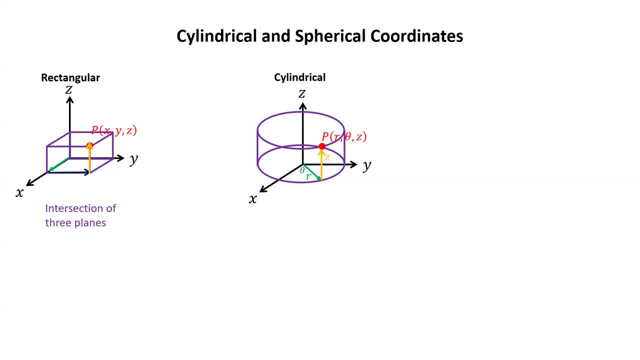 the same point. We can replace theta by theta plus any multiple of 2 pi and we get the same point. Another way to get the same point would be to use a negative r value and to adjust theta by pi To guarantee that there's only one way to write the point. we'll insist. 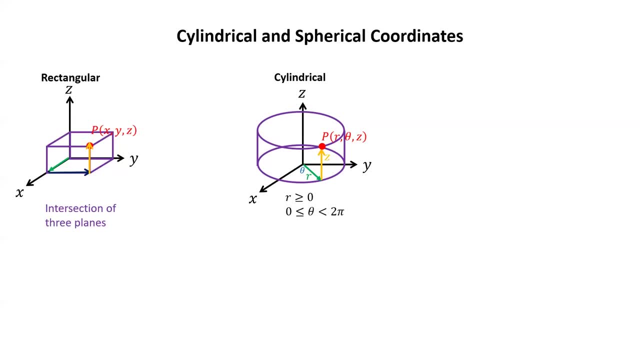 when we write down a point that r is non-negative and theta is between 0 and 2 pi. 0 can be used, 2 pi should not be used, because if theta is 0 or theta is 2 pi, you would get the same point. 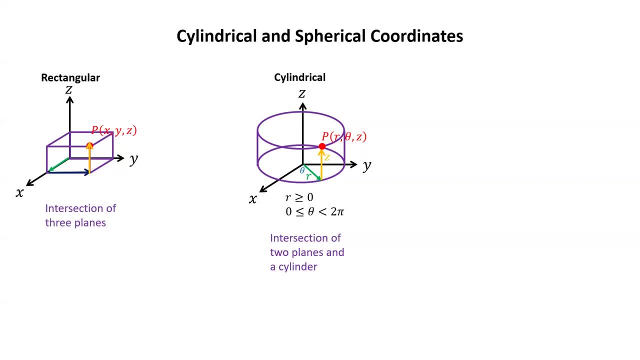 Notice that when you think of a point in cylindrical, you're thinking of it as the intersection of two planes and a cylinder. The cylinder has equation: r equals some value, Just like in rectangular. the z coordinate leads to a plane and the theta coordinate also leads to a plane, the plane that starts with the z-axis. 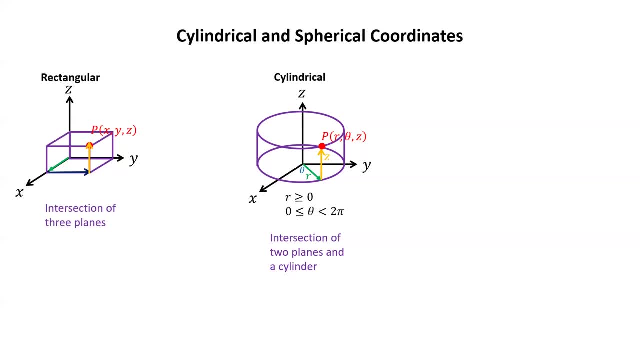 and comes straight out along the ray that is determined by theta. In spherical, our points have the form rho theta phi. We could think of our point as lying on a sphere. To get to the point, we come straight out from the origin: rho units. 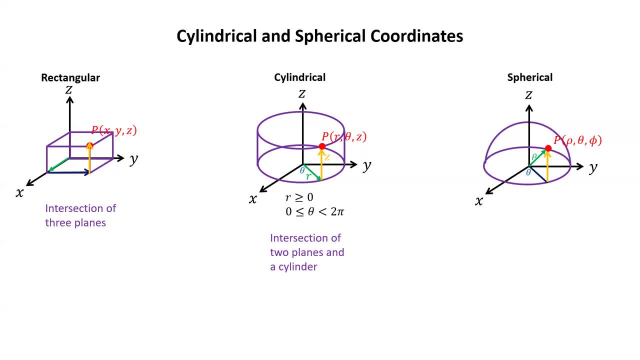 theta is the same theta that we use in cylindrical. It's the angle in the x-y plane that we make with the positive x-axis, and phi is the angle that we make with the positive z-axis, Just like in cylindrical, since there are infinitely many ways to write down a given point. 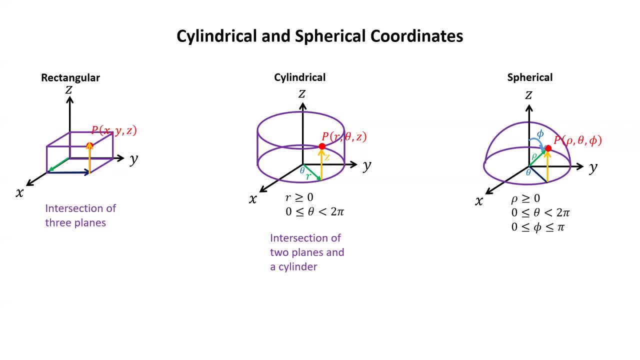 we could make that unique by insisting that rho is non-negative, theta is between 0 and 2 pi, including 0. And phi should be between 0 and pi. In the case of phi, we include both 0 and pi, A point that has. 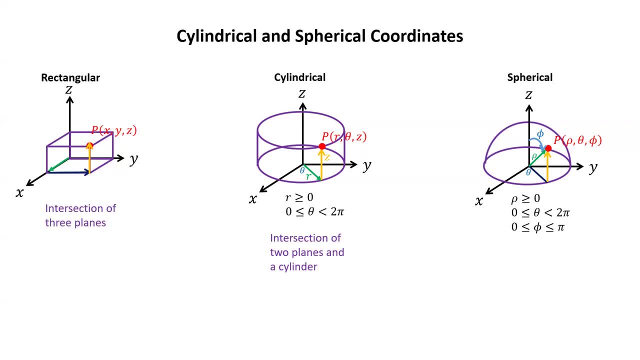 a phi coordinate of 0 is on the positive z-axis. A point that has a phi coordinate of pi is on the negative z-axis. Just to give one more example: if the phi coordinate is pi over 2, then the point will be in the x-y plane. It's halfway between the positive z-axis and the negative z-axis. 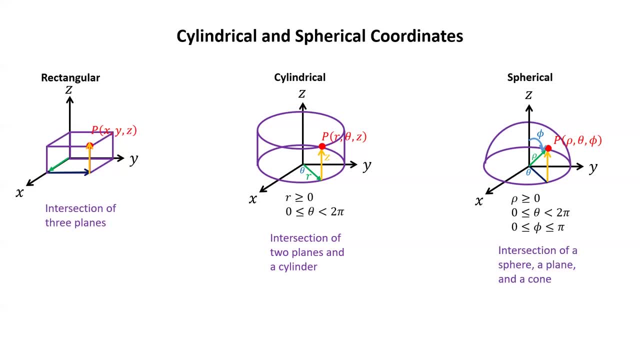 Note that when we plot a point in spherical, we're thinking of it as the intersection of a sphere, a plane and a cone. The sphere is given by the rho coordinate, The plane is given by the theta coordinate, just like in cylindrical, and the cone is given by the phi coordinate. 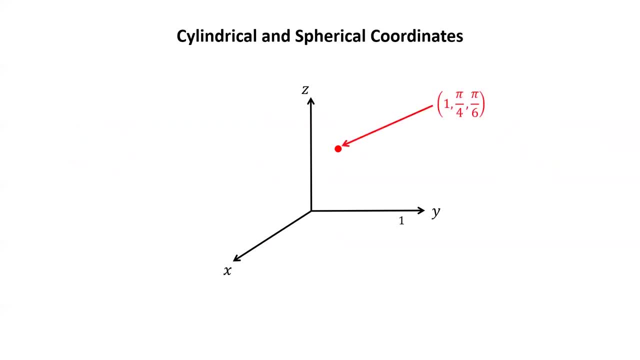 To help clarify what I just said, let's look at a specific point like 1, pi over 4, pi over 6.. We're thinking of this as in spherical, so rho is 1, theta is pi over 4, and phi is pi over 6.. Since rho is 1, we know that the point lies on a sphere. 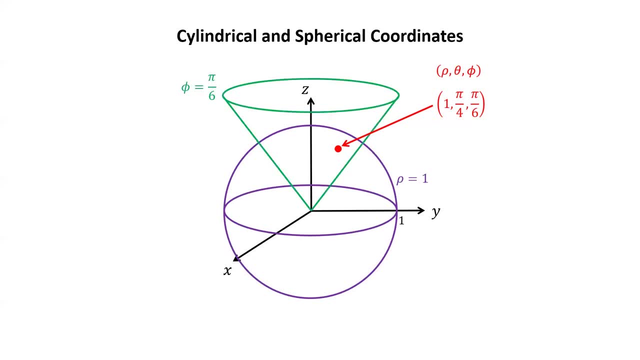 of radius 1 centered at the origin. Since phi is pi over 6, we know that the point lies on a cone that makes an angle of pi over 6 from the positive z-axis. Notice that the intersection of the sphere and the cone is this circle, So our point lies on this circle that is the intersection of the. 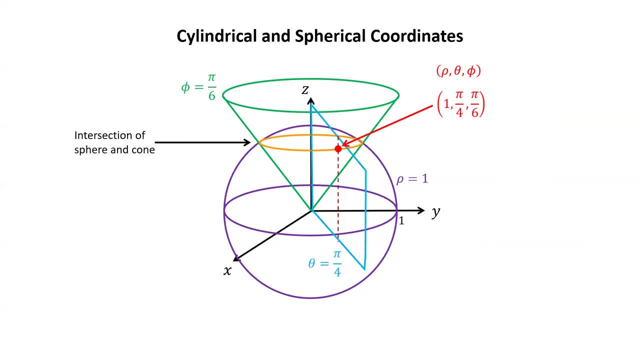 given sphere and cone, The plane defined by theta equals pi over 4 intersects that circle in a unique point. Now let's learn how to convert points between the various coordinate systems, starting with converting between rectangular and cylindrical. Here we have a point written. 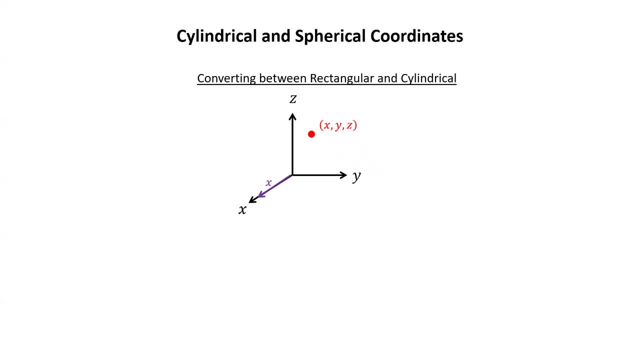 in rectangular as x, y, z, which means we go x units along the x-axis, y units parallel to the y-axis and z units perpendicular to the y-axis. So we're going to convert the points along the x-y-plane. Now, if we want to think of that same point in cylindrical, then we're going to go. 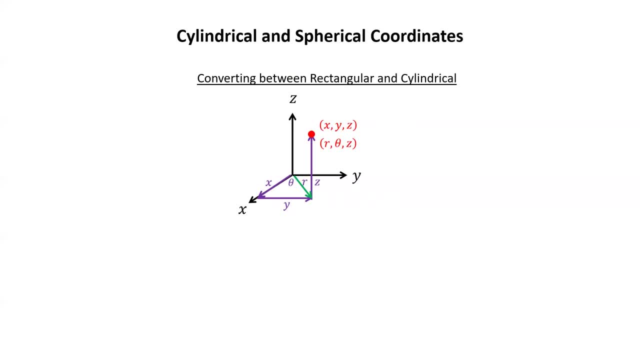 straight out in the x-y-plane from the origin r units, making an angle of theta with the positive x-axis, And then we go straight up z, just like we did in rectangular. Let's just look at that triangle that was formed in the x-y-plane. Notice that in the x-y-plane we go. 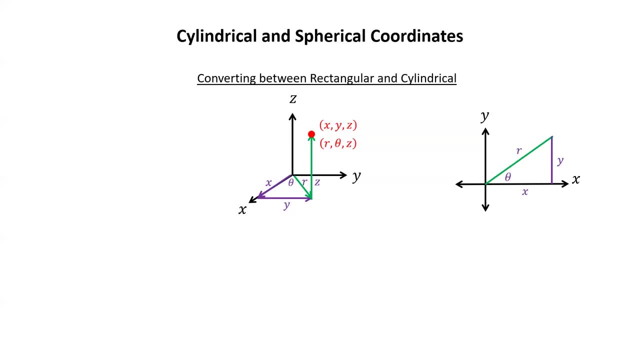 x units along the x-axis and then y units parallel to the y-axis. to get to the point, if we're thinking of it in rectangular, Or we go straight out from the origin, r units making an angle of theta with the positive x-axis. if we're thinking of it in cylindrical, 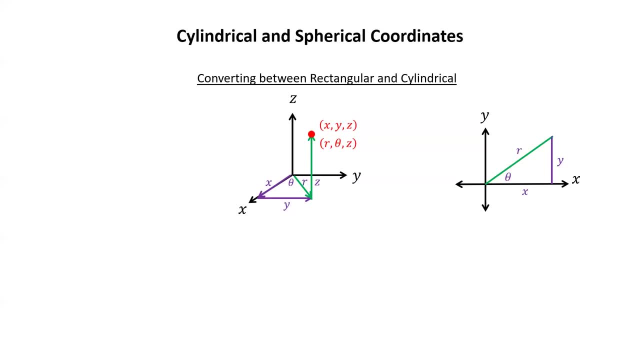 Or we could think of that as polar in this case, since we changed the picture to a two-dimensional picture. Notice that x is equal to r cosine theta and y equals r sine theta. just from basic trigonometry. These are the same things that we did in the x-y-plane, So we're going to go straight out. 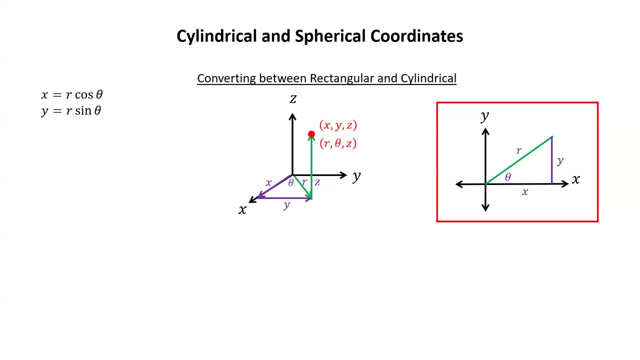 the same transformations we have for polar coordinates, And similarly, x squared plus y squared is r squared and the tangent of theta is y over x. Again, that's from basic trigonometry of the right triangle, or just remembering that those are the polar transformations. 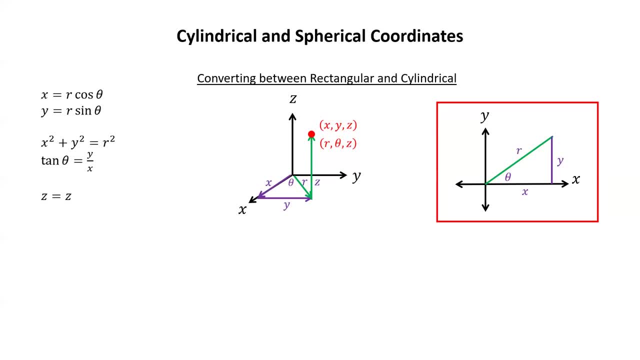 Finally, z is just equal to z. In other words, we're using the same z value for both rectangular and cylindrical. Let's try a couple of examples. Go ahead and pause the video, try these examples yourself and then resume the video to check your answers with mine. 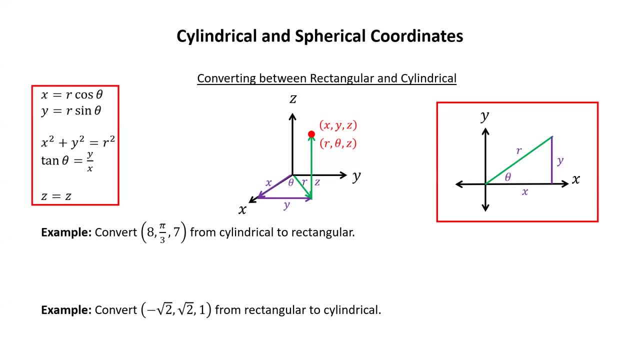 First convert 8, pi over 3,, 7 from cylindrical to rectangular. Okay, so we're thinking of 8 as the r coordinate, pi over 3 as the theta coordinate and 7 as the z coordinate. So the x coordinate is: 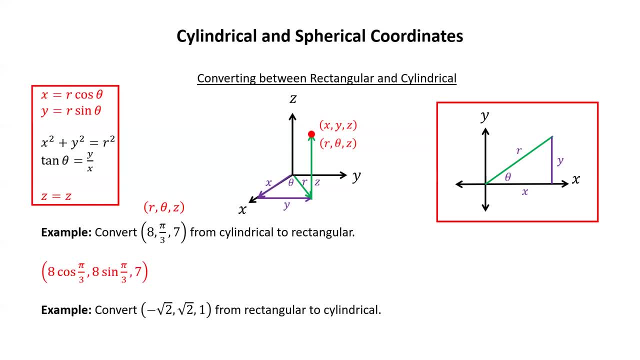 8 cosine pi over 3, the y coordinate is 8 sine pi over 3, and the z coordinate is 7.. So the cosine of pi over 3, that's 1.. 1 half, 8 times 1 half, is 4.. The sine of pi over 3 is root 3 over 2.. 8 times root 3 over 2 is 4. 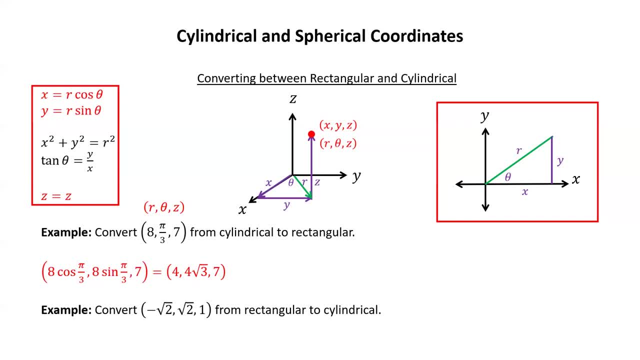 root 3.. And we'll leave the 7 as is. So we get 4, 4 root 3, 7.. So x is 4, y is 4, root 3, and z is 7.. Let's look at the second example. Convert negative root 2, root 2, 1 from rectangular to cylindrical. 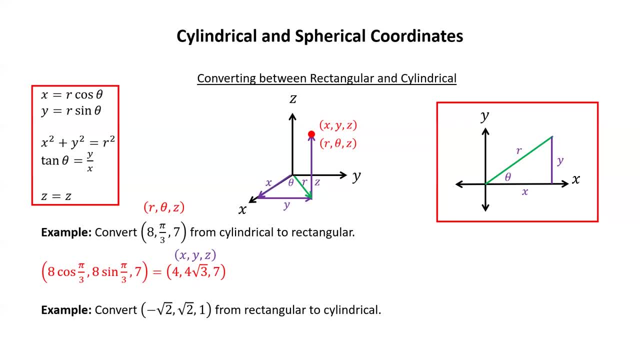 So in this case, x is negative root 2,, y is root 2, and z is 1.. Let's just look at the projection of this point in the xy plane. So we're just looking at negative root 2, root 2.. To plot the: 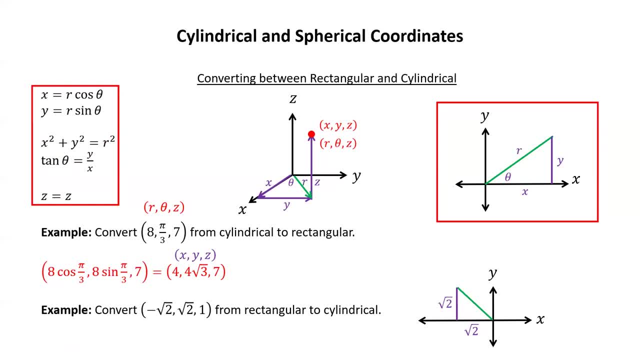 point, negative root 2, root 2 in the xy plane. we go left- root 2, because the x-coordinate is negative, and then up root 2.. From there it's pretty easy to convert. r is the square root of. 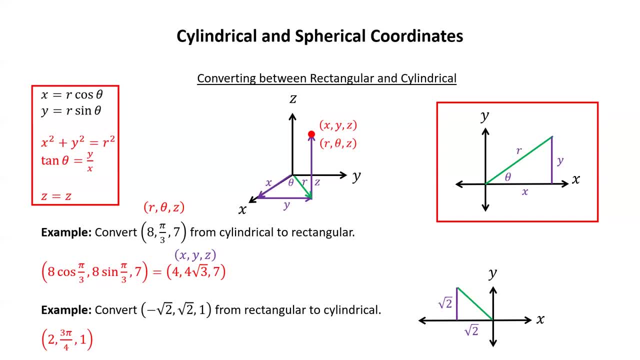 root 2 squared plus root 2 squared, or the square root of 2 plus 2, or 4.. So the square root of 4 is 2.. Theta is the angle formed with the positive x-axis, So the reference angle that's inside that triangle would be pi over 4.. And therefore theta is pi minus pi over 4,. 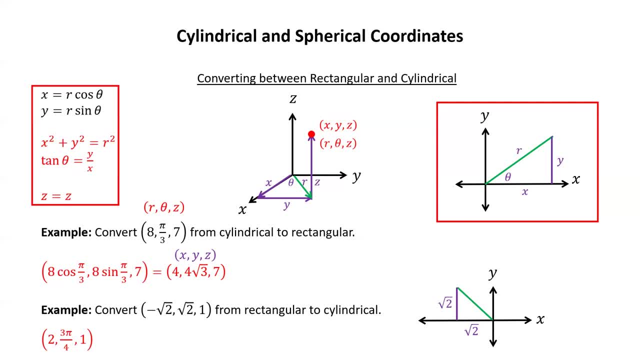 which is 3 pi over 4.. And the z-coordinate is the same as the z-coordinate in rectangular, So we just put a 1 there. So the point is 2, 3 pi over 4, 1.. Now let's go over how to convert. 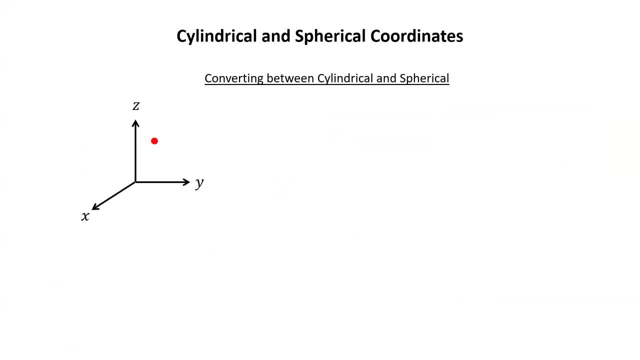 between cylindrical and spherical. So here we have a point. In cylindrical, its coordinates are r, theta, z, which means we come out r units in the xy plane, making an angle of theta with the positive x-axis, and then go straight up z units. Now let's see what we do in spherical, In spherical. 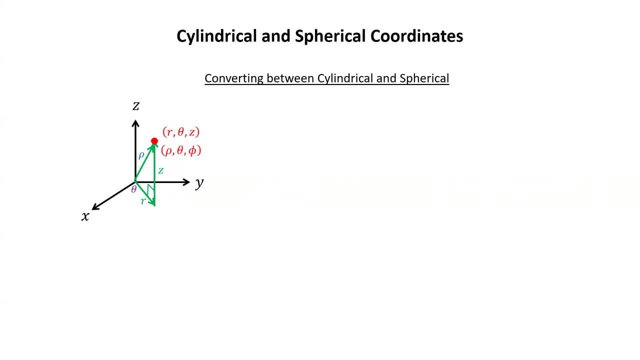 we're going to come straight out from the origin to the point row units and we're going to come down from the positive z-axis with an angle Of phi. Theta is the same Now, using the fact that when you have two parallel lines cut by a 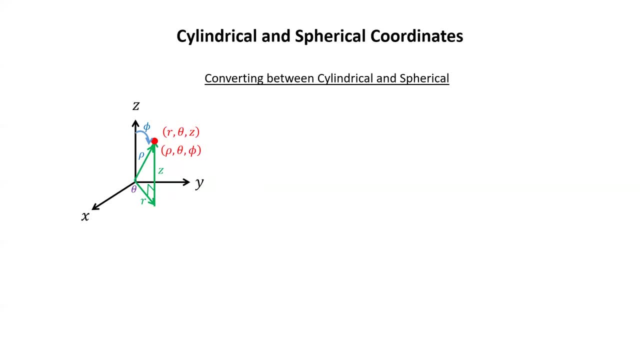 transversal. the alternate interior angles are congruent. we see that we could write phi inside the triangle, the angle between the sides of lengths rho and z. Let's just look at that triangle for a minute. Notice it's a right triangle. We drew it a little funny here because it's being 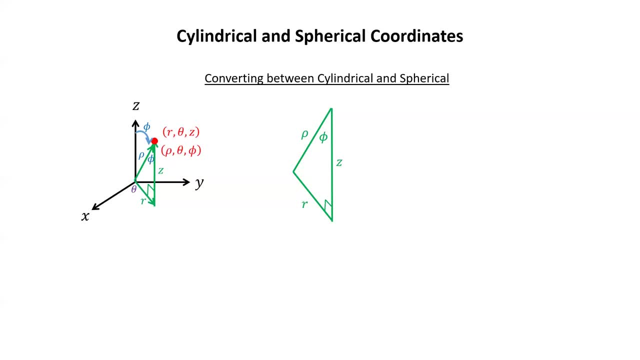 drawn in three dimensions. But if you look at this triangle, its behavior is exactly the same as the triangle We drew for converting between rectangular and cylindrical, or rectangular and polar. We have r equals rho sine phi and z equals rho cosine phi, again using basic trigonometry of the right. 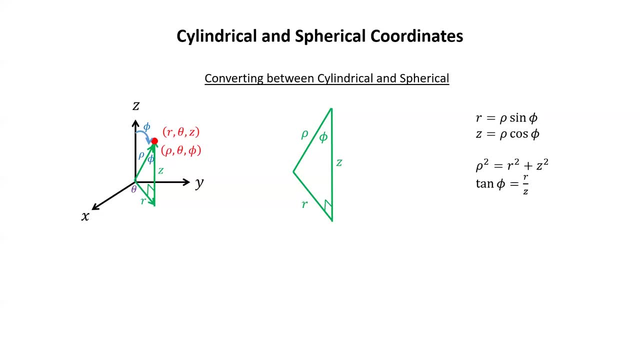 triangle, Rho squared is r squared plus z squared. Once again, pay attention to where that right angle is. It looks a little funny because it's drawn in three dimensions, but that angle is a right angle. And we have tan phi is r over z because tangent is opposite over adjacent, And 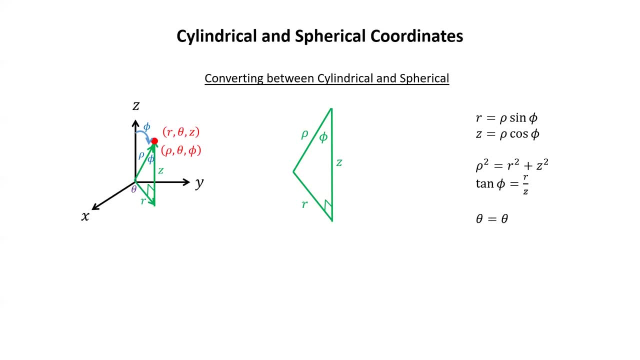 finally, theta equals theta. We're using the same theta for both cylindrical and spherical In practice. you can memorize these formulas, or you could just remember how to draw this picture. I prefer to just draw that triangle each time I need to make these conversions rather than have to memorize the formulas. That said, 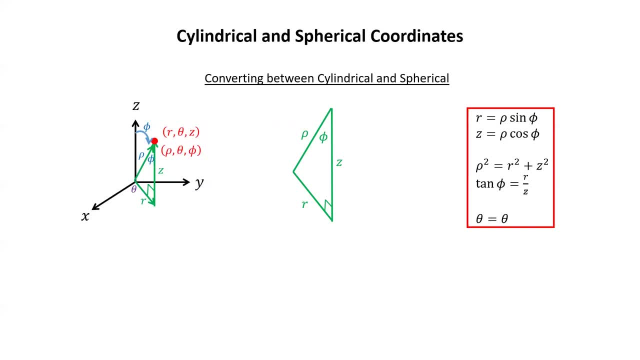 notice that the formulas are identical to the formulas for converting between rectangular and cylindrical, except all the names of the variables have been changed. Okay, go ahead and try this example. Pause the video. Try it yourself first and then resume the video to check your answer with mine. 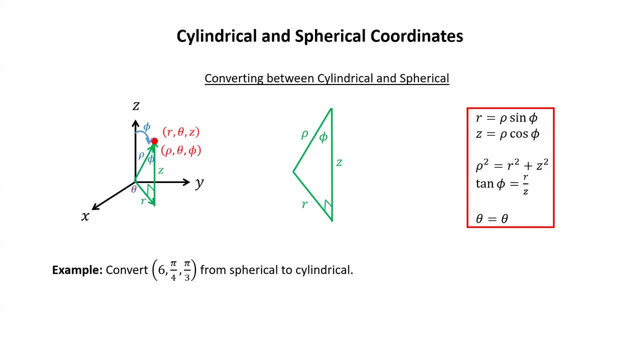 Okay, let's convert six, pi over four, pi over three from spherical to cylindrical. Notice that six is the rho coordinate, pi over four is the theta coordinate and pi over three is the phi coordinate. Let me draw the picture. So rho is six in that picture and phi is pi over three in that picture. 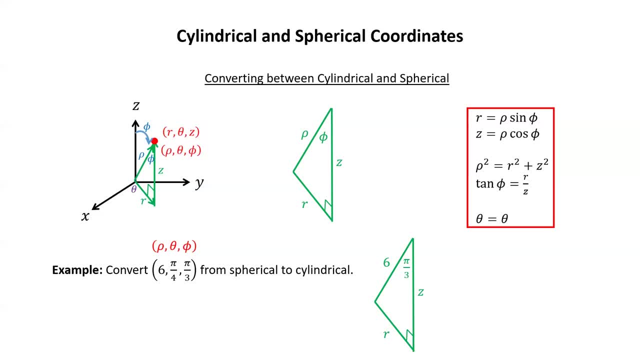 Notice I don't have to draw theta in the picture, because theta is going to be exactly the same. We can just copy it over. Using the picture and some basic trigonometry or just plugging directly into the formulas, we get that r is rho sine phi, which is six. 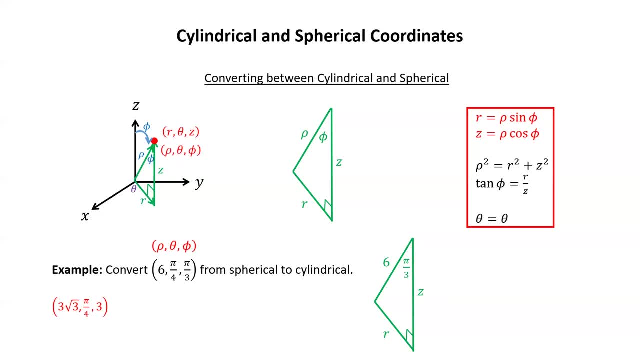 sine pi over three, which is six times root three over two, or three root three, The theta coordinate we just copy over, that's pi over four, And for z we get rho cosine phi, which is six. cosine pi over three, which is six times one half, or pi over four, And for z we get 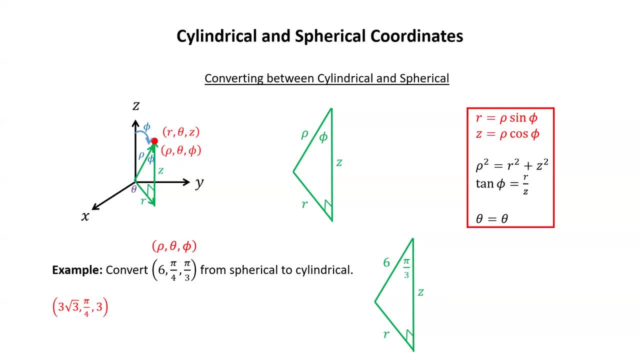 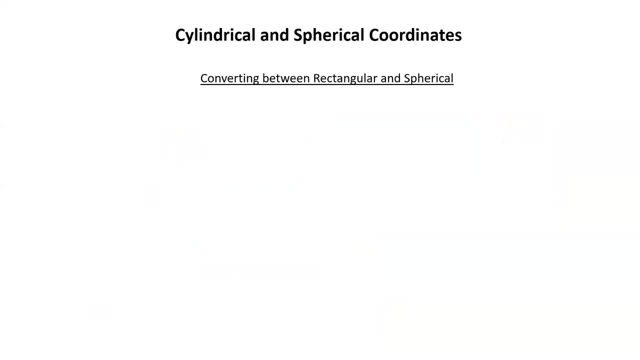 zero cosine, pi over three, which is six times one, half or three. So the point in cylindrical is three root three, pi over four, three. And now finally, let's go over converting between rectangular and spherical. There are two ways we can convert between rectangular and spherical. 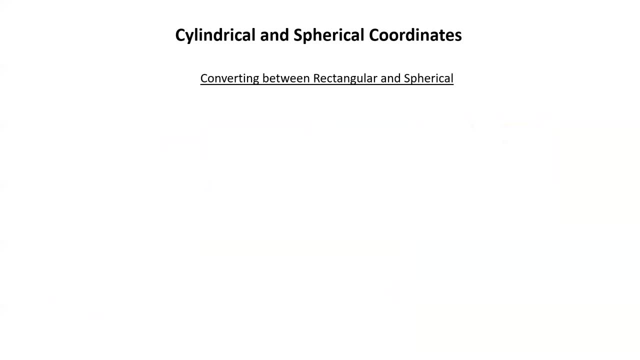 First way is just to use cylindrical. For example, if we want to convert from rectangular to spherical, we can convert from rectangular to cylindrical first and then from cylindrical to spherical. And similarly, if we want to convert from to rectangular, we could convert from spherical to cylindrical and then cylindrical to rectangular. 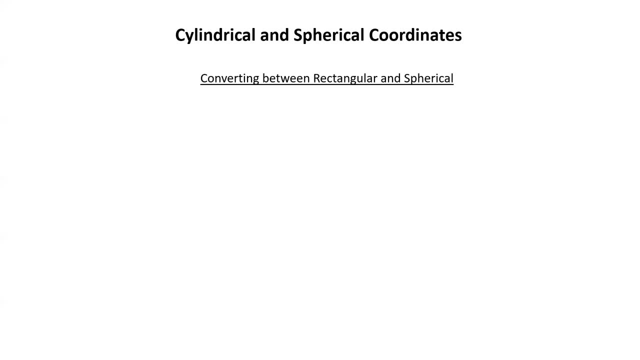 That said, I'm going to show you what direct formulas you get if we copy that procedure in general. So here's a picture of the triangle that we have for converting between cylindrical and spherical, And writing down the formulas for converting between rectangular and cylindrical. 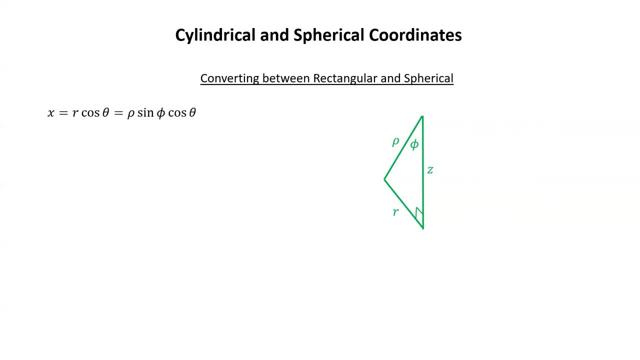 we have x equals r cosine theta, And if you look at the picture you could see that r is equal to rho sine phi. So we have x is rho sine phi cosine theta. Similarly, y equals r sine theta And again, r is rho sine phi. So y is rho sine phi sine theta. To get z, you could either use: 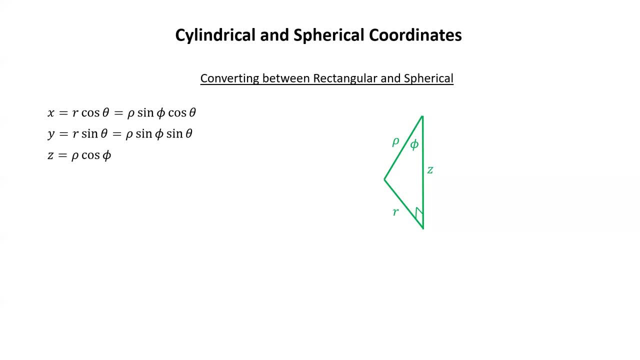 the picture or if you have the formulas memorized from converting between cylindrical and spherical, we know that it's just z is rho cosine phi. For the other direction from the picture or the conversions between cylindrical and spherical, we have rho squared is r. 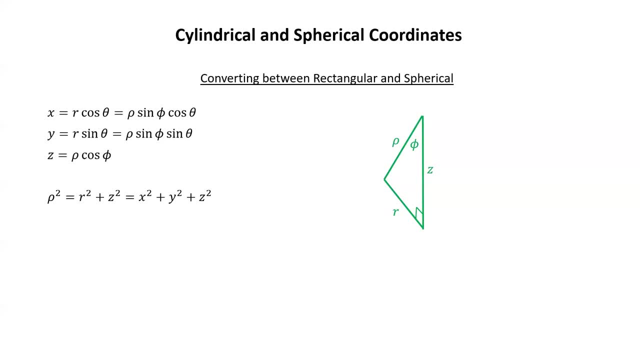 squared And if you look at the picture, you could either use the picture or if you have z squared but r squared is x squared plus y squared. So rho squared is x squared plus y squared plus z squared. Tangent of theta is y over x And cosine phi is z over rho, But rho is the. 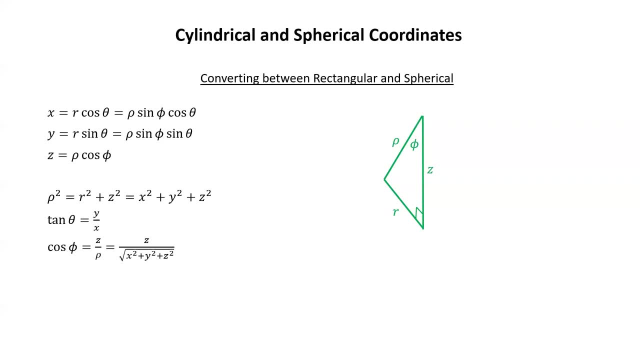 square root of x squared plus y squared plus z squared. So cosine phi is z over the square root of x squared plus y squared plus z squared. Okay, let's try some examples of converting between spherical and rectangular. Pause the video, try these yourself and then resume the video to. 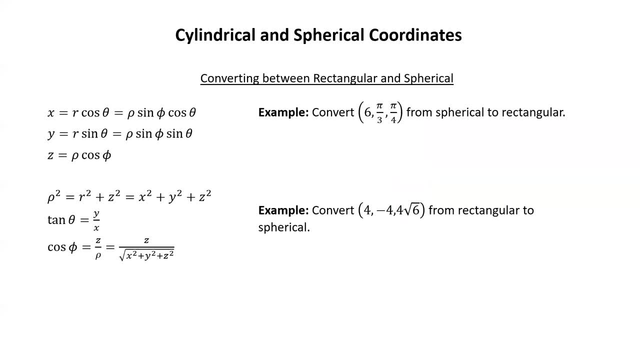 check your answers with mine. First one convert six pi over three, pi over four, from spherical to rectangular. Okay, just plugging into the formulas: x is rho sine phi cosine theta, So that's six sine pi over four, cosine pi over three. Y is rho sine phi sine theta, So that's six sine pi over. 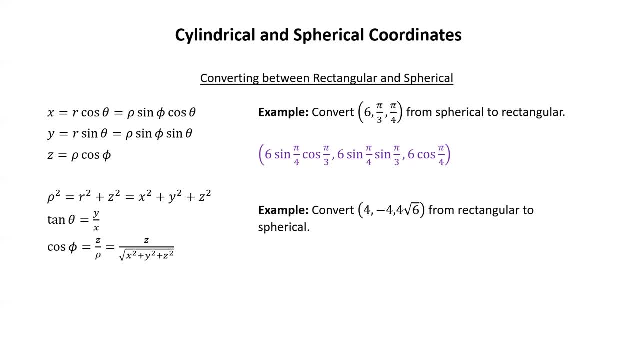 four sine pi over three, And z is rho cosine phi. So that's six cosine pi over four, And our final answer is three root two over two. three root six over two, three root two. Now convert four negative four, four root six from rectangular to spherical. Let's draw a picture of 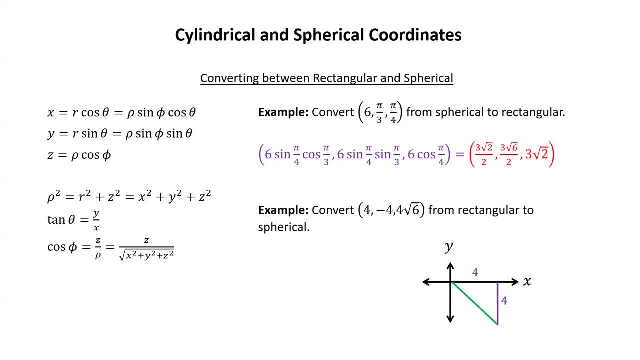 the projection of the point into the xy plane. So we're just looking at the point. four, negative four. in the xy plane We go right. four down four. We go down instead of up because the y coordinate there is negative. So from this picture we see that the angle theta is negative. 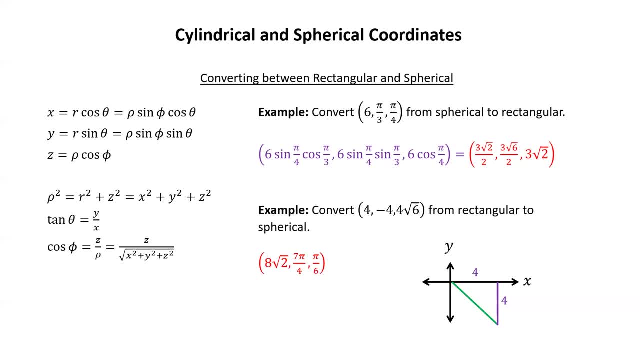 The angle theta is seven pi over four. We get that by taking two pi minus the reference angle of pi over four. right, Two pi minus pi over four is seven pi over four. And we could get rho by taking the square root of x squared plus y squared plus z squared, So that's the square root of four. 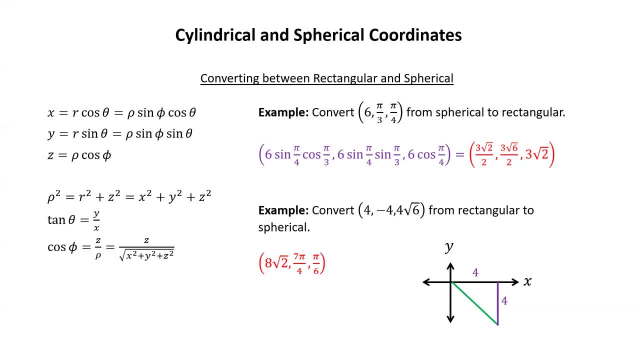 squared plus the square of negative four plus four root six squared, which comes out to eight root two. And finally we could get the phi coordinate by seeing that cosine of phi is z over rho Z is six. Rho we just found to be eight root two. So taking the inverse cosine of that gives us pi over. 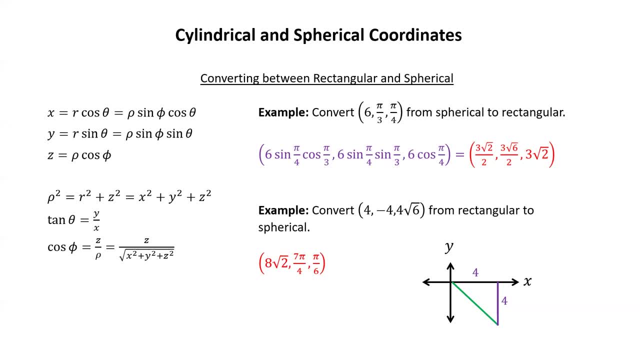 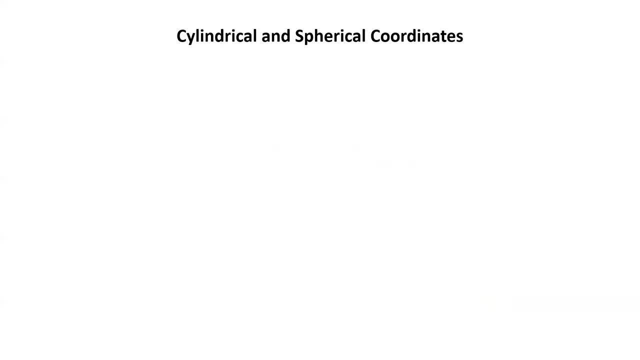 six. You may want to check all those computations carefully yourself. Let's finish up this section by looking at the equations of some familiar surfaces in all three coordinate systems. Let's start with a cone. Specifically, let's start with the cone. z equals the square root of x. 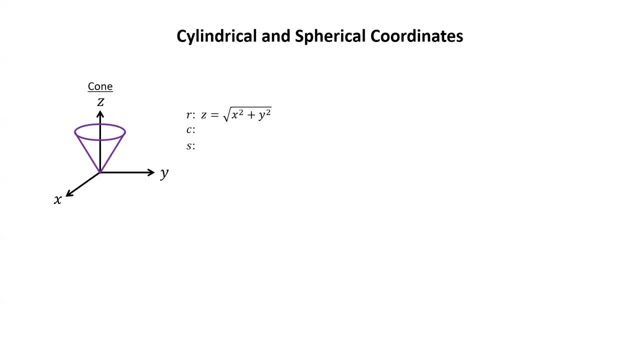 squared plus y squared. Technically, this is just the upper half of the cone, Since I'm only looking at the positive square root. pause the video. try to write these equations in cylindrical and spherical and then resume the video to check your answers. Remember that to 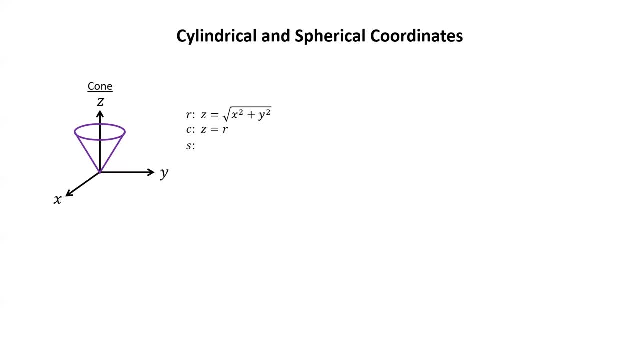 convert between rectangular and cylindrical. we could use the formula r squared as x squared plus y squared. So we get the square root of x squared plus y squared is the square root of r squared, which is just r. So we have z equals r in cylindrical. Now to convert that equation: 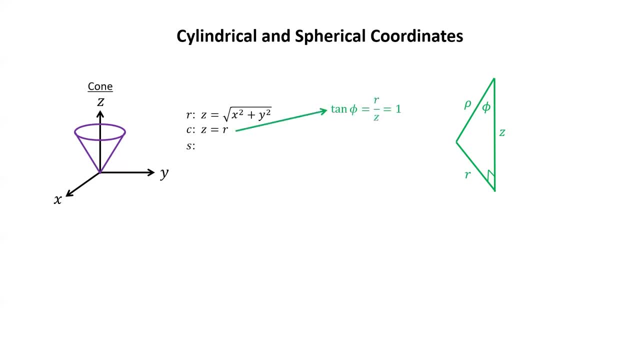 from cylindrical to spherical. we could use our triangle here. Notice that r over z is equal to 1.. And using either that picture or if you have the formulas memorized, we see that the tangent of phi is r over z, which in this case is 1.. So that phi is equal to pi over 4.. So this cone in spherical 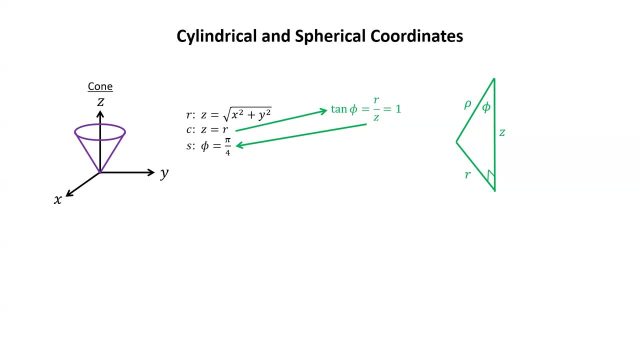 is the constant function. phi equals pi over 4.. Next, let's try a basic cylinder. Let's use the unit cylinder In rectangular. that is equation: x squared plus y squared equals 1.. Once again pause the video. try to write this equation in cylindrical and spherical as well. 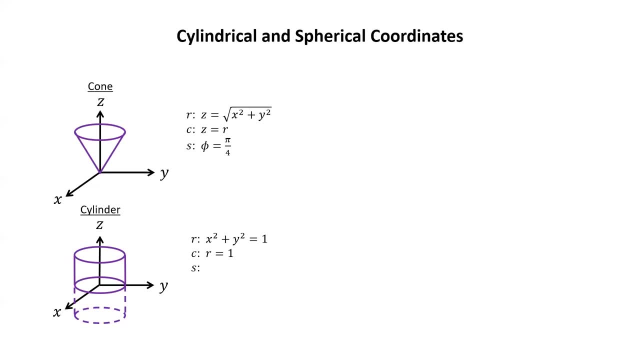 Then resume the video to check your answer with mine. For cylindrical, since x squared plus y squared equals r squared, we have r squared equals 1 or, equivalently, r equals 1.. For spherical, we see that the sine of phi is equal to r over rho And since r is 1, we have the sine of phi.